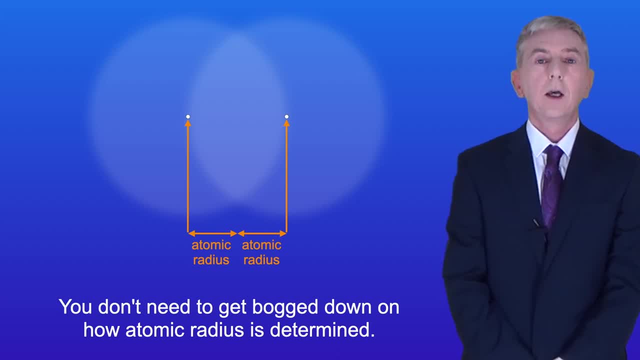 Now you don't need to get bogged down on how atomic radius is determined, but you need to understand that we cannot measure the radius of an atom directly, as electron clouds do not have a clear cut-off point. However, one way of calculating atomic radius- 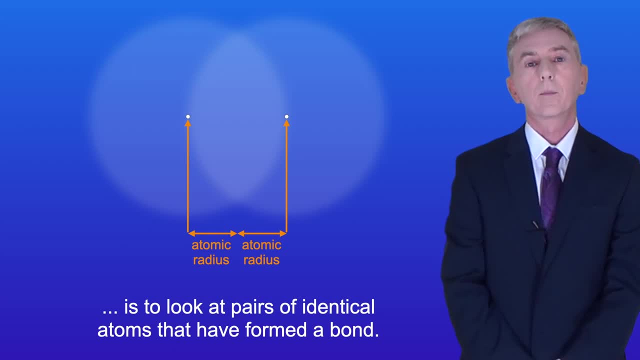 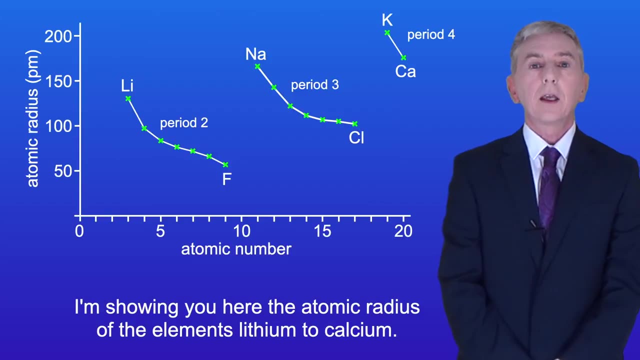 is to look at pairs of identical atoms that are formed to bond. We take the atomic radius as half the distance between the nuclei of the two atoms. I'm showing you here the atomic radius of the elements lithium to calcium. You'll notice that I haven't included the noble gases, as they don't take part in. 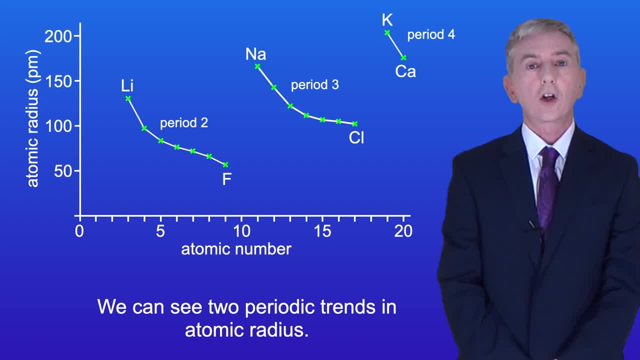 bonding, We can see two periodic trends in atomic radius. Firstly, atomic radius decreases as we move across a period from left to right. So looking at period two, we can see atomic radius decreasing from lithium to fluorine. and looking at period three, 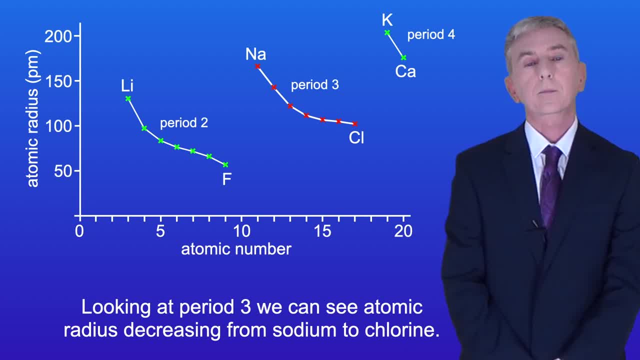 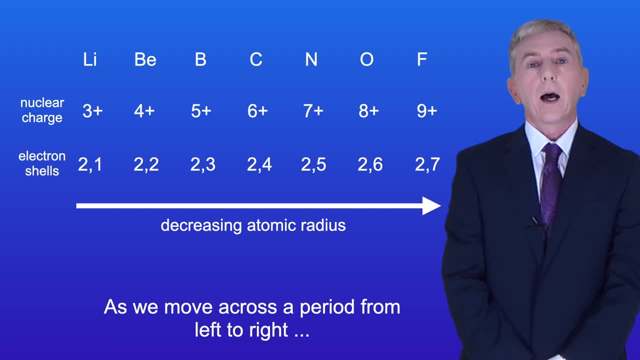 we can see atomic radius decreasing from sodium to chlorine. I'm going to explain this by looking at period two, but this applies to the other periods. As we move across a period from left to right, each element has one more proton in its nucleus than the element before. 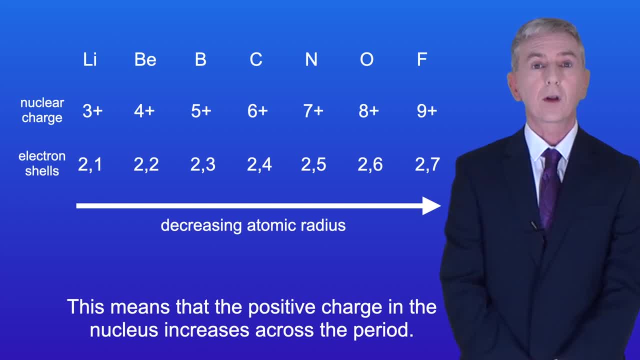 This means that the positive charge in the nucleus increases across the period. Because of this increased positive charge, there's an increased attraction between the nucleus and the electrons and this draws the electrons closer to the nucleus. This causes the atomic radius to decrease across the period. Remember that outer shell electrons are partially shielded. 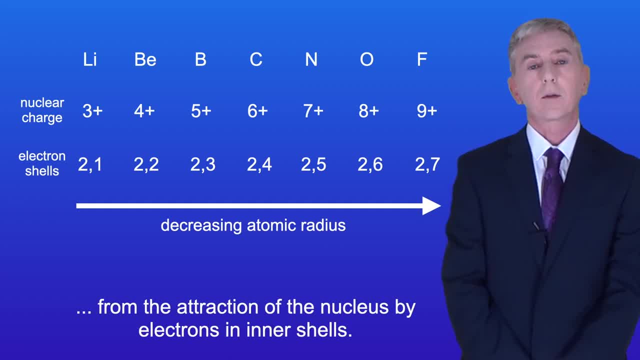 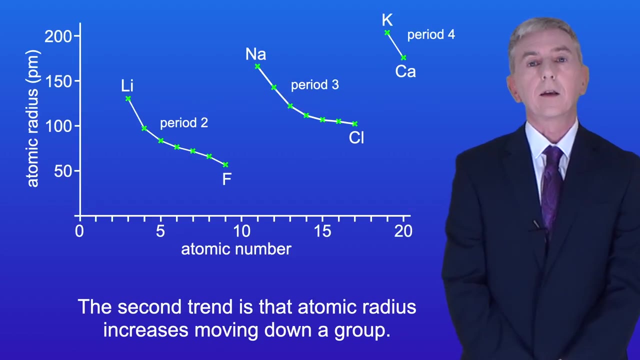 from the attraction of the nucleus by electrons in inner shells. However, all of the elements in period two only have one inner electron shell, So this means that shielding due to the inner electrons is not possible. Now the second trend is that atomic radius increases, moving down a group. We can see: 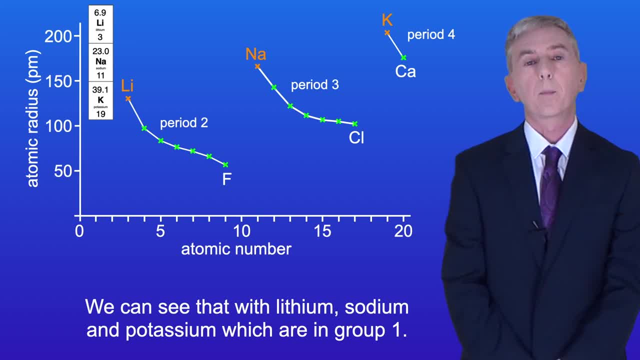 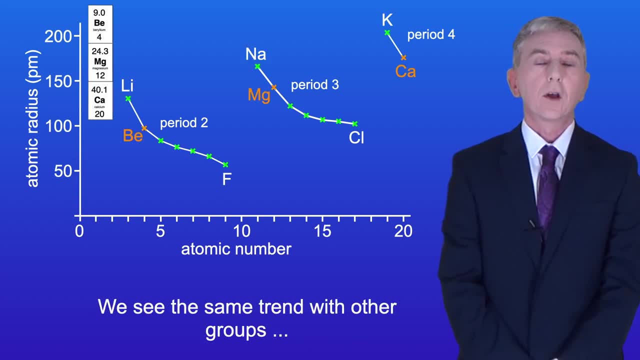 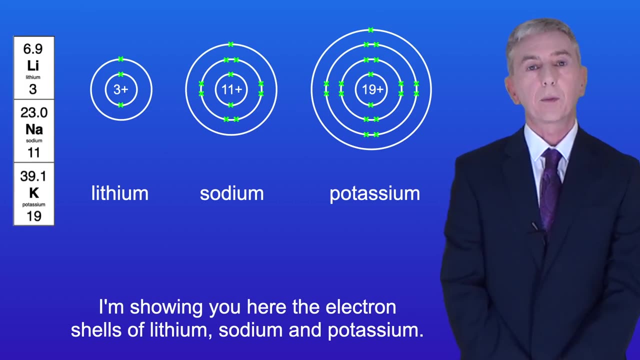 that with lithium, sodium and potassium, which are in group one, As we move down group one, atomic radius increases. We see the same trend with other groups, for example group two, which we can see here. I'm showing you here the electron shells of lithium, sodium and potassium. The number: